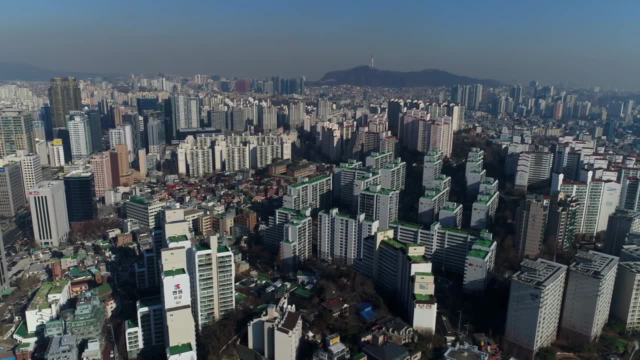 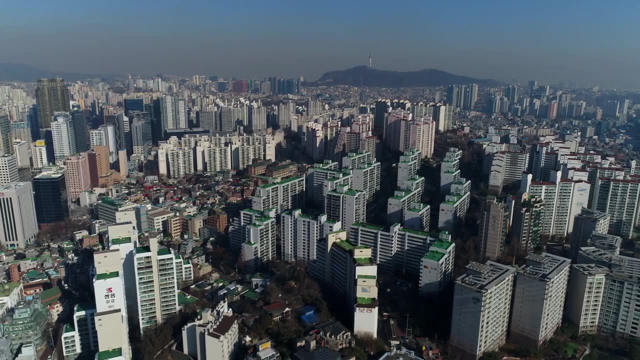 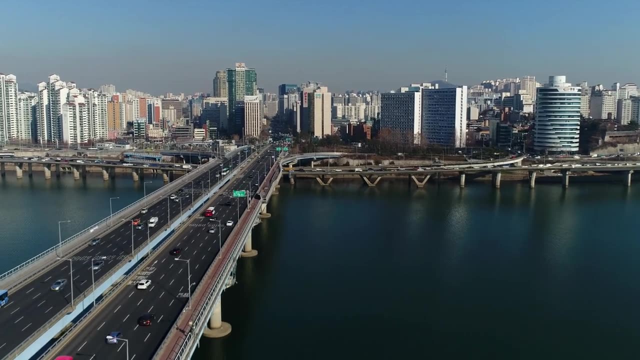 The only non-European nation in the top five. South Korea had a recycling rate of 53.7% in 2018.. It has enjoyed success until now with a system in which privately run companies collect the waste and sell it on for profit. However, this is due to change soon after near-neighbor China. 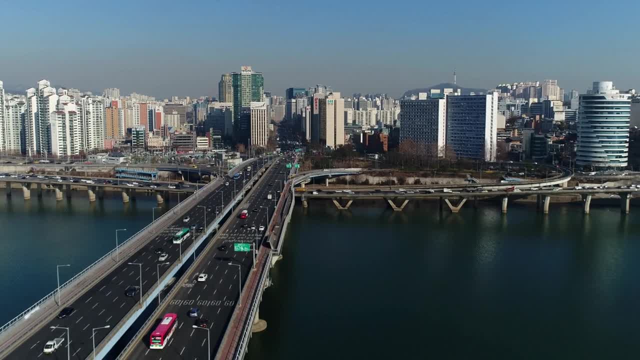 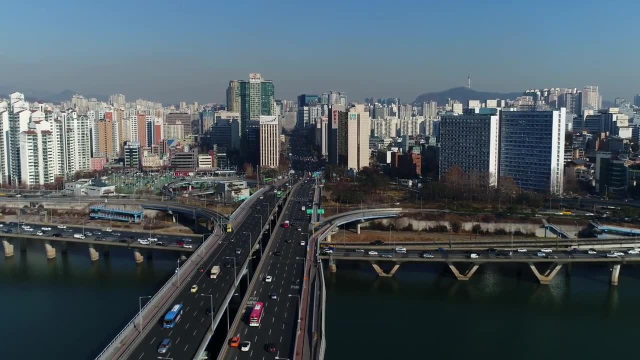 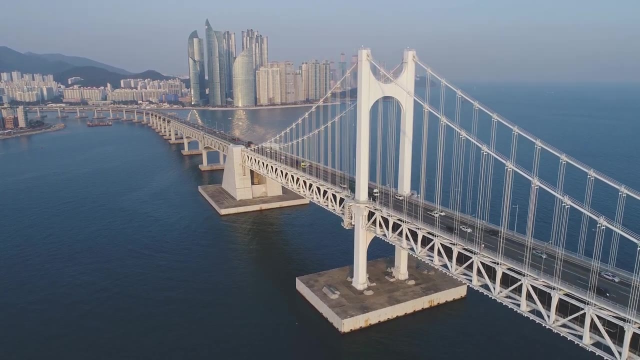 altered its own environmental policy. In April last year, the economic superpower banned the import of plastic waste and, as the biggest buyer of Korean material, this was a problem. Last year, China banned the import of plastic waste, causing Korean recycling companies to lose significant amounts of money. 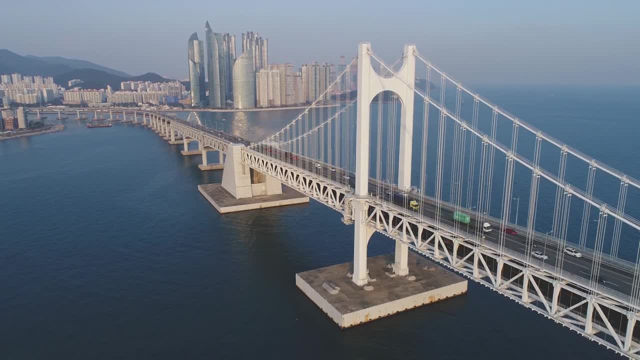 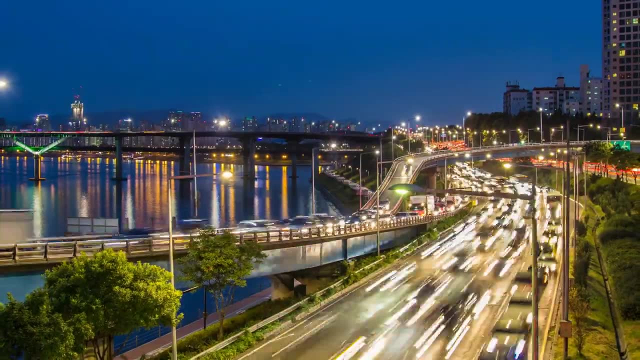 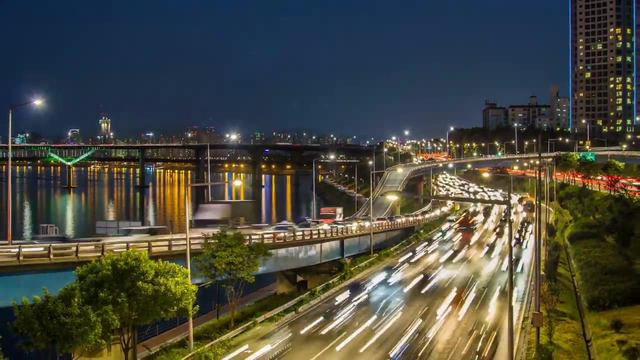 Korean business. Businesses are no longer making as much money from the recycling scheme, resulting in staff lay-offs and plastic waste starting to pile up on its streets. These issues lasted for two weeks before the government agreed to provide financial help to the recycling companies. Commenting on the waste management crisis. former Environment Secretary. 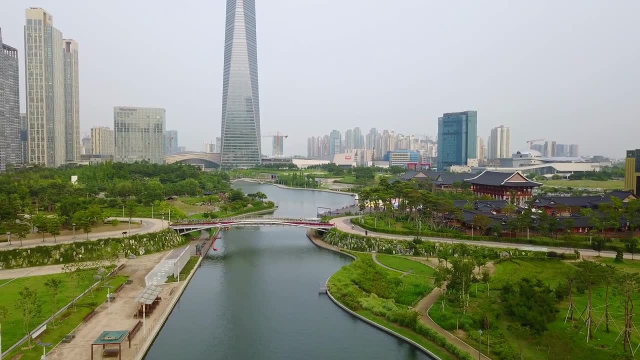 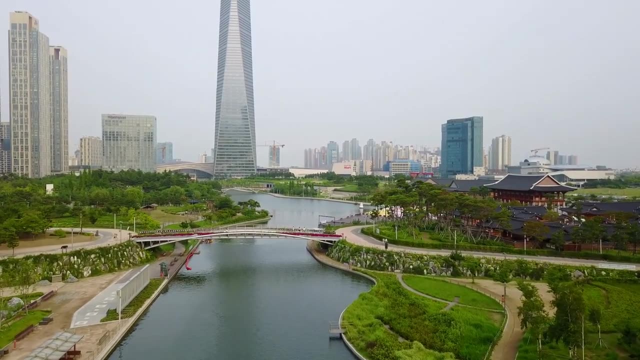 Kim Eun-kyung said, To resolve the plastic waste crisis, society as a whole needs to change its ways of production, consumption, recycling and even the culture. South Korea has since implemented policies that include the banning of both coloured plastic bottles and PVC by 2020.. 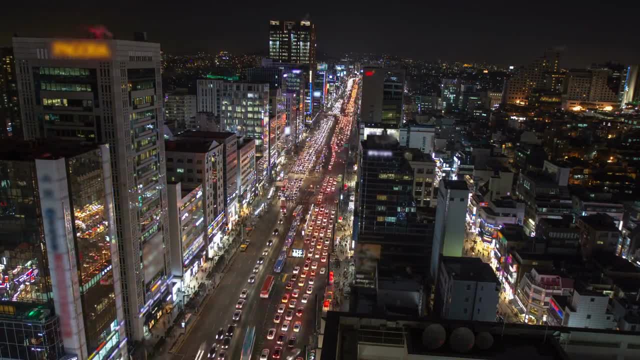 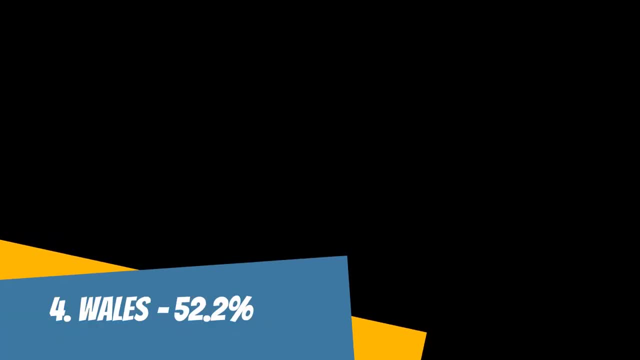 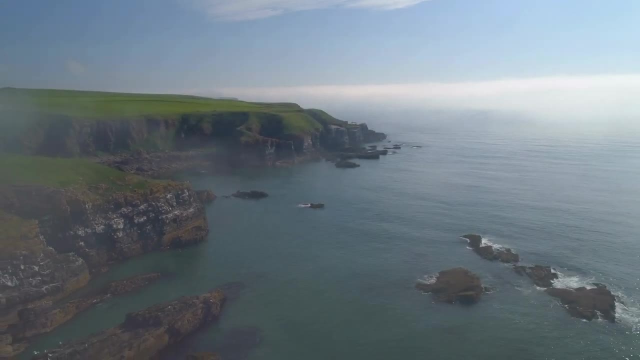 It will also reduce and eventually phase out disposable cups and plastic screws, getting rid of these products completely by 2027.. 4. Wales- 52.2%. Wales has a constitutional responsibility for promoting sustainability. It's the smallest country on the list, but Wales is flying high when it comes to its 52%. 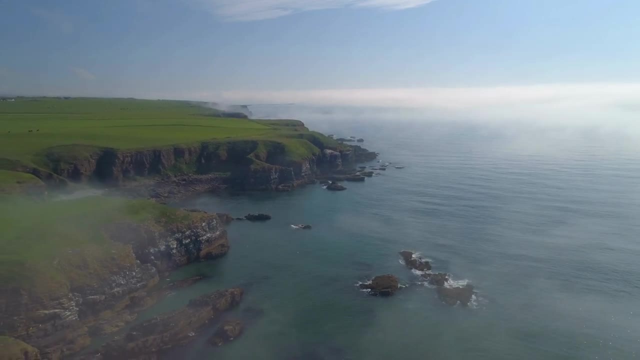 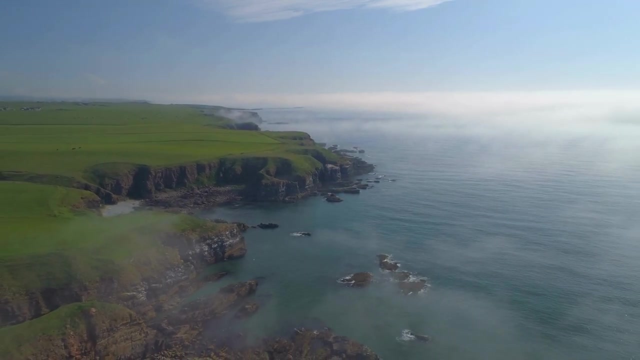 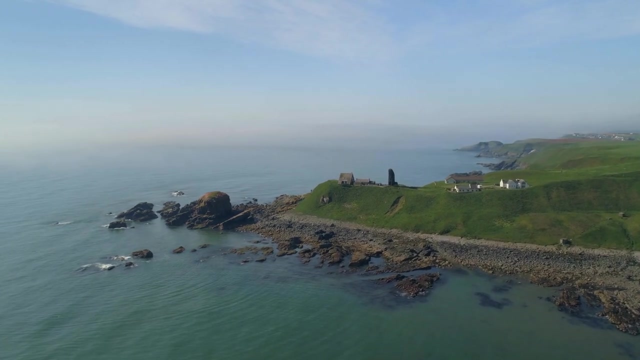 recycling rate recorded in 2018.. Due to constitutional rules set out by the country's devolved government, its policymakers have a statutory duty to help promote sustainable development. Like the rest of the UK, recycling in Wales is operated by local administrations. However, the Welsh Assembly has offered a recovery system to local areas that can. 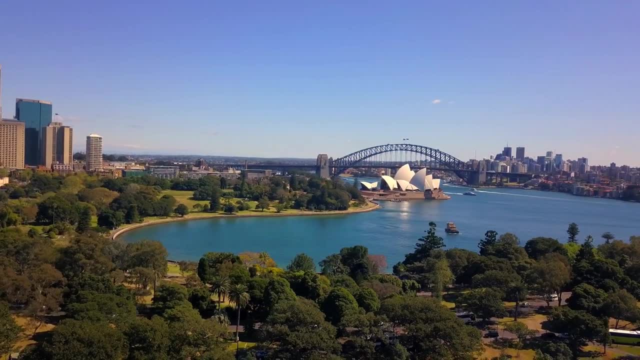 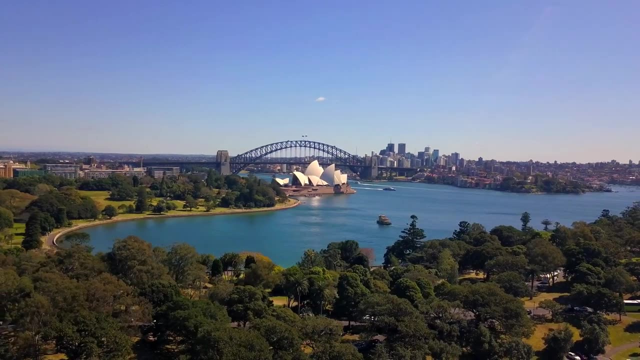 be financed by councils, with most taking the scheme on board. This means that both people and businesses have similar rules on what can and can't. This means that the economy of Wales can't be recycled across the country. Alongside this, Wales operates a circular economy in all but name, according to Dr Andy Rees.